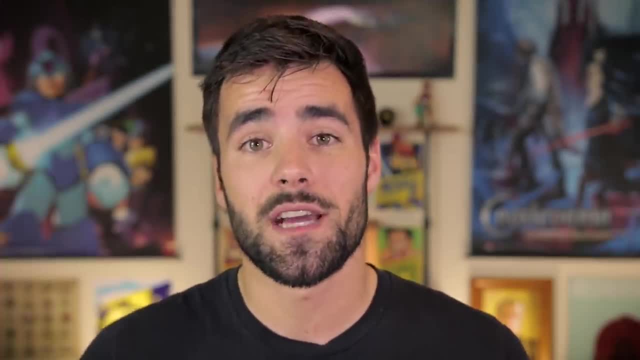 the course of studying math and working through these tough problems, you are eventually going to come to problems that just stump you, that you get completely stuck on, And when you get to these points, it's important to know how to eventually solve these problems and 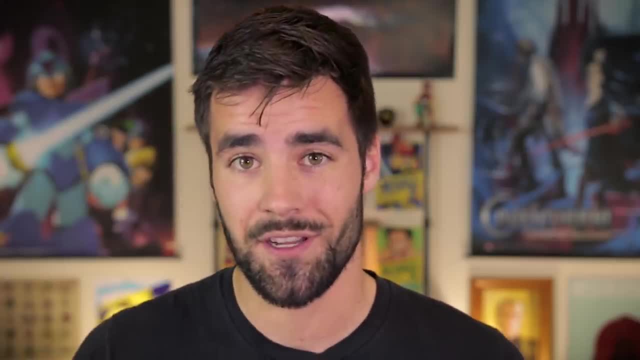 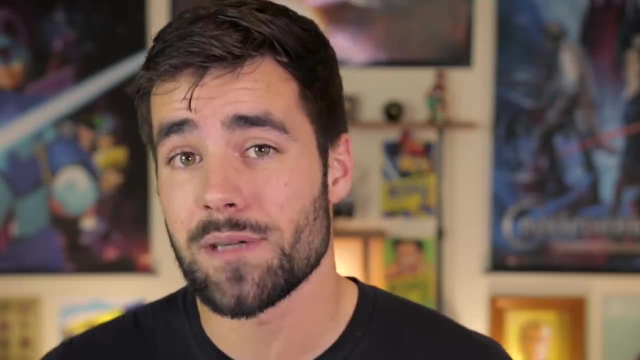 these are the ones that are really going to stretch and build your skill set. So that is what I want to focus on in this video. I want to give you some practical techniques for working through and eventually solving those problems that seem insurmountable at 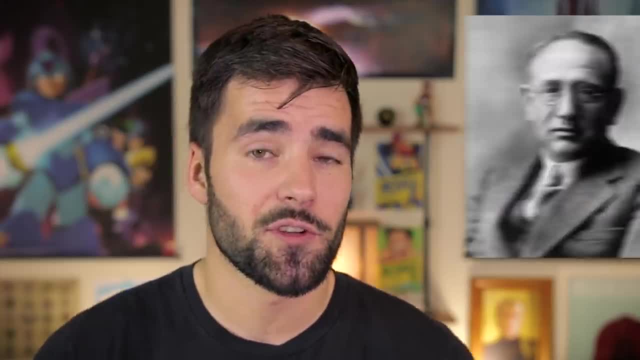 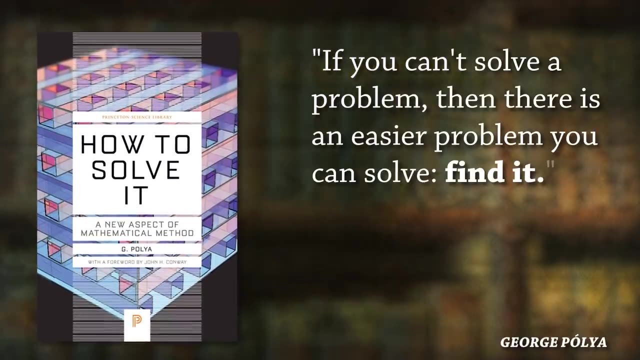 first To start, I want to focus on a piece of advice that the Hungarian mathematician George Poya shared in his 1945 book How to Solve It. It goes: if you can't solve a problem, then there is an easier problem that you can solve. Find it. This is, in my opinion, the 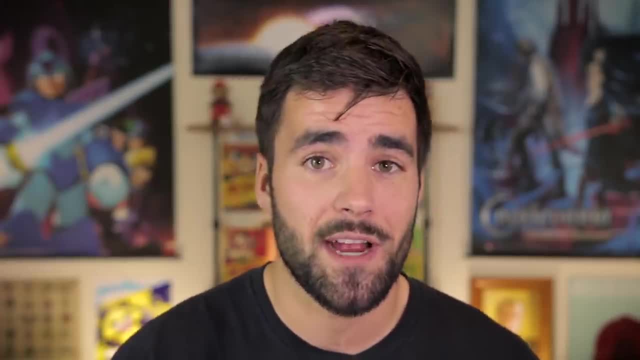 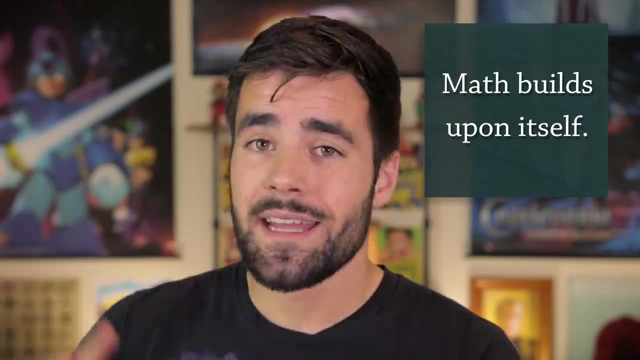 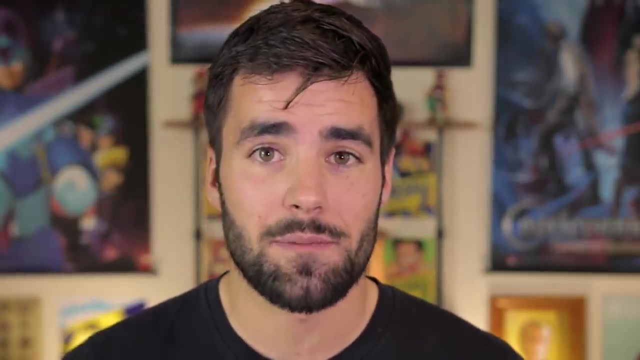 most important technique to understand and put into practice when you're trying to solve tough math problems, Because math builds upon itself. More complex concepts are built upon simpler concepts And if you don't have a strong grasp on the fundamental principles then a more complex problem is going to likely stump you. So if you come across a problem, 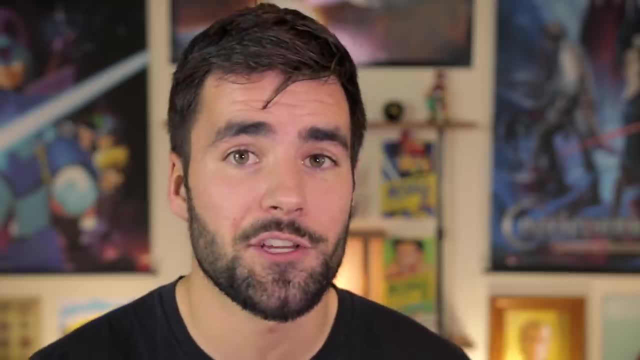 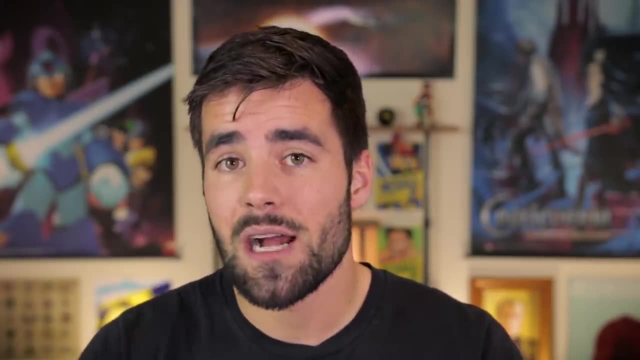 that you can't solve. first identify the components or the operations that it wants you to carry out. A lot of times, complex problems will have multiple. Now what you can do in this case is split the problem into multiple problems that isolate just one of those components. 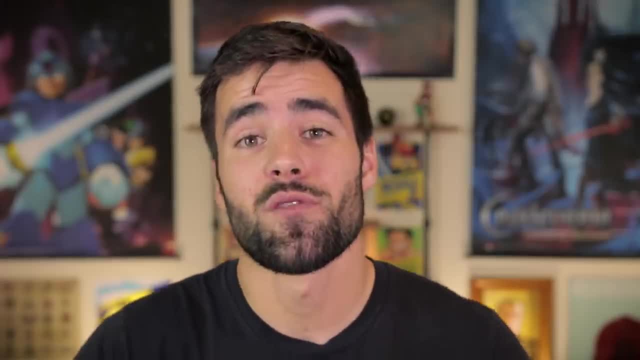 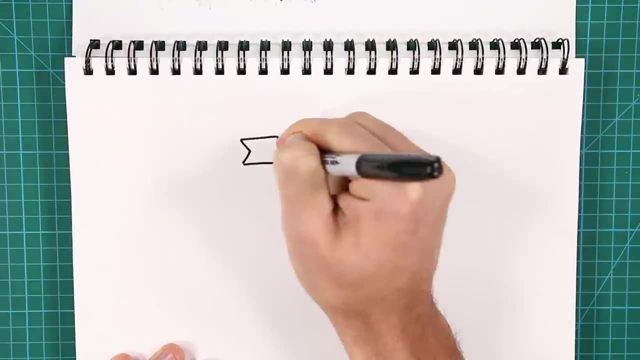 or operations. So I want to show you this concept in action. so let's work through a quick example. Now I did have one example picked out that would be pretty easy, but it ended up being a little bit too easy, so let's do something a little bit more complicated. So this is a summation. 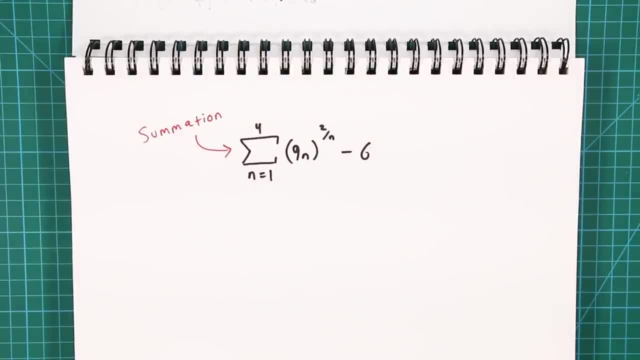 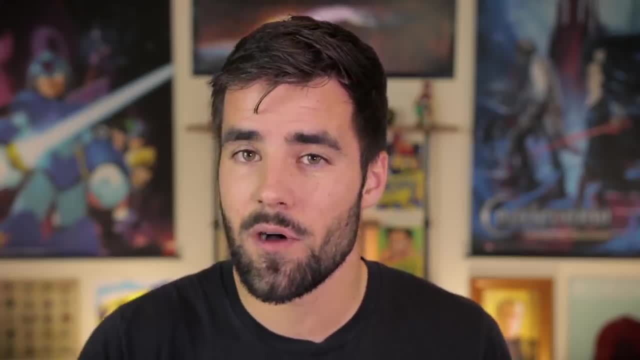 problem which uses the Greek symbol sigma, And it essentially says that we're going to add up a series of expressions that use a variable, starting at one and ending at four, But if you notice, this summation problem also has a fractional exponent in it. Now, 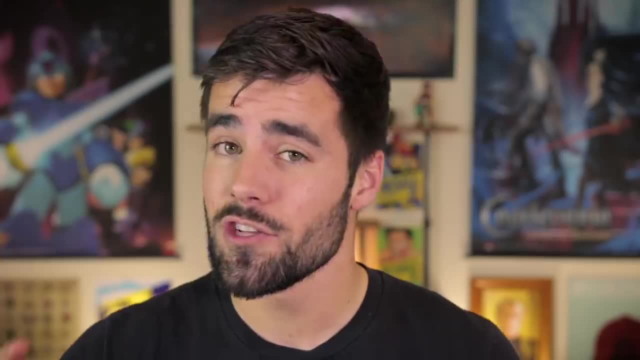 maybe some of you math wizzes out there could do this kind of a problem in your sleep, but it's also possibly the case that you don't have a really good idea of how to solve a really firm grasp on either summation or fractional exponents. So when you're working, 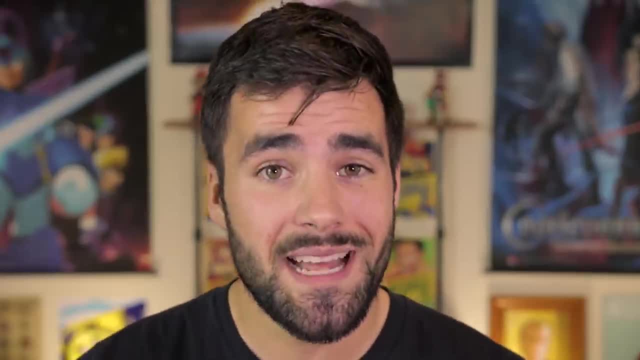 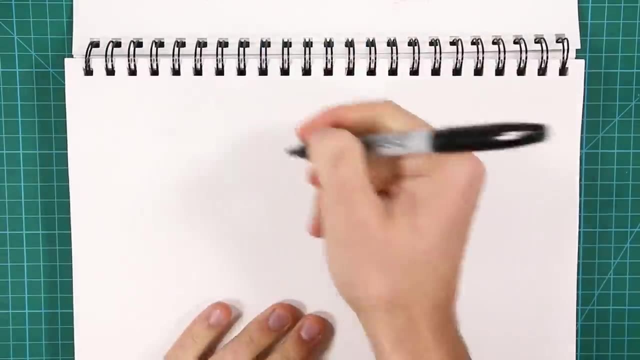 a problem that combines the two of them, you might get stuck. So, assuming that's the case, let's break this problem into two simpler problems that each focus on just one of the underlying concepts. First, let's create a simpler summation problem that just gets rid. 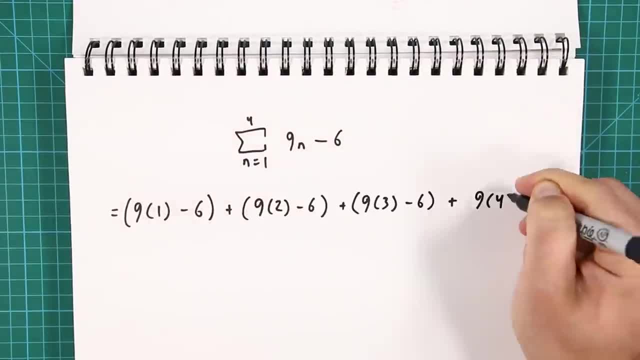 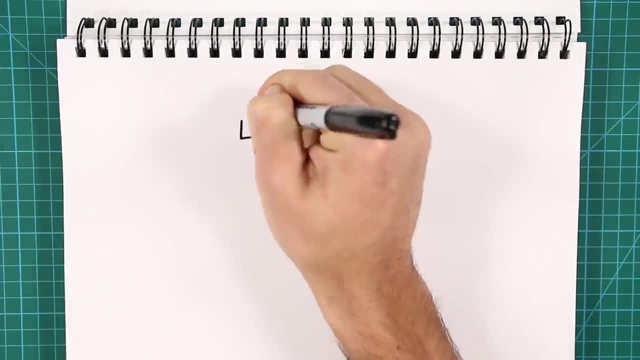 of that fractional exponent altogether. Now all we have to do is evaluate that expression four times and then add up the answers, which gets us to a final answer of 66.. And now let's move on to the fractional exponent. Now I'm going to go pretty quick here, because this: 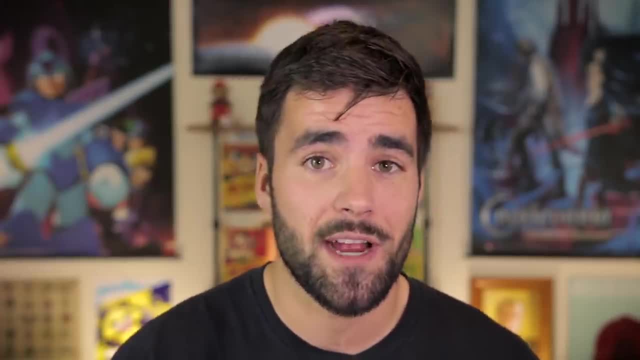 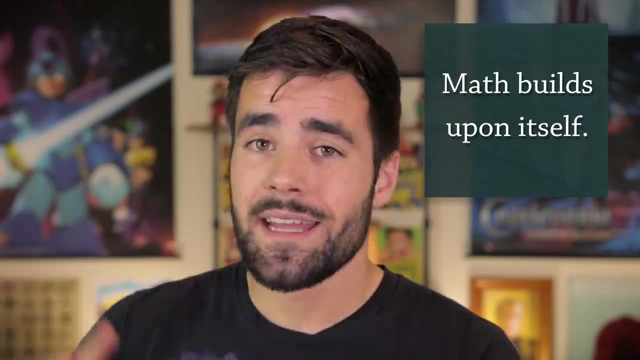 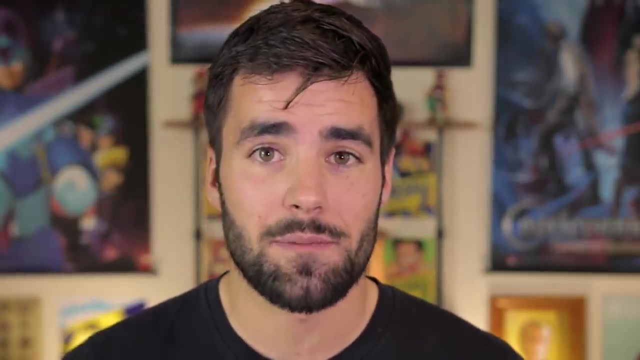 most important technique to understand and put into practice when you're trying to solve tough math problems, Because math builds upon itself. More complex concepts are built upon simpler concepts And if you don't have a strong grasp on the fundamental principles then a more complex problem is going to likely stump you. So if you come across a problem, 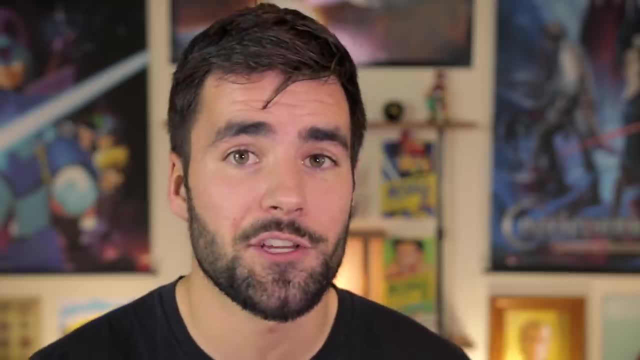 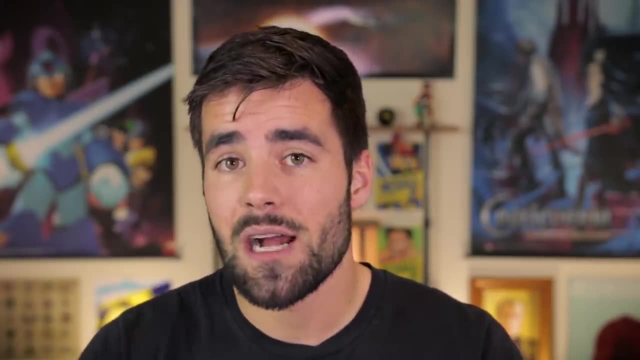 that you can't solve. first identify the components or the operations that it wants you to carry out. A lot of times, complex problems will have multiple. Now what you can do in this case is split the problem into multiple problems that isolate just one of those components. 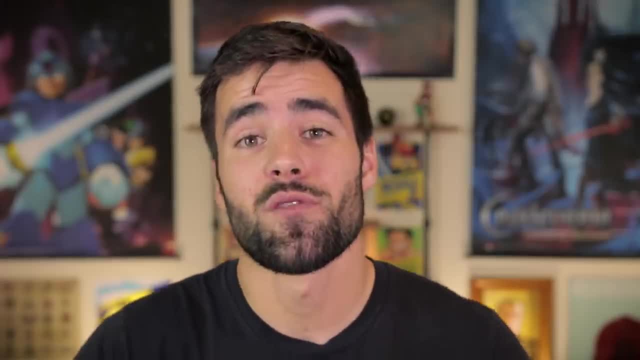 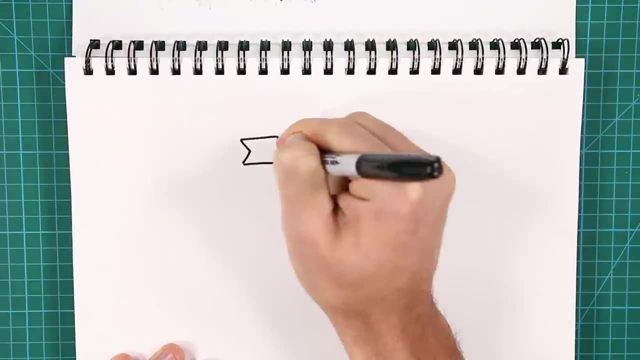 or operations. So I want to show you this concept in action. so let's work through a quick example. Now I did have one example picked out that would be pretty easy, but it ended up being a little bit too easy, so let's do something a little bit more complicated. So this is a summation. 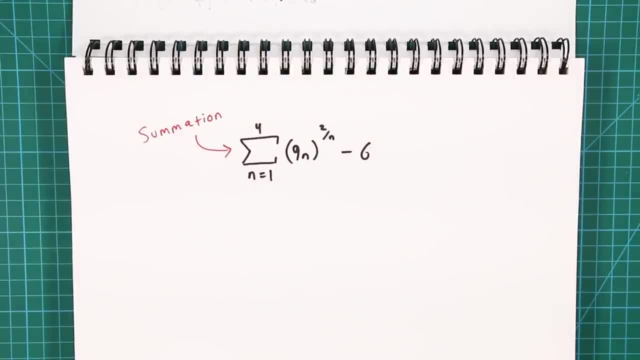 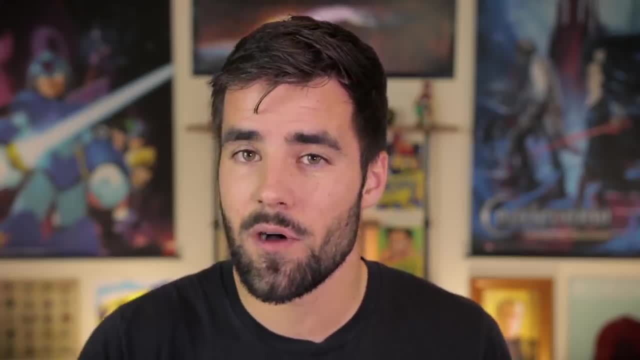 problem which uses the Greek symbol sigma, And it essentially says that we're going to add up a series of expressions that use a variable, starting at one and ending at four, But if you notice, this summation problem also has a fractional exponent in it. Now, 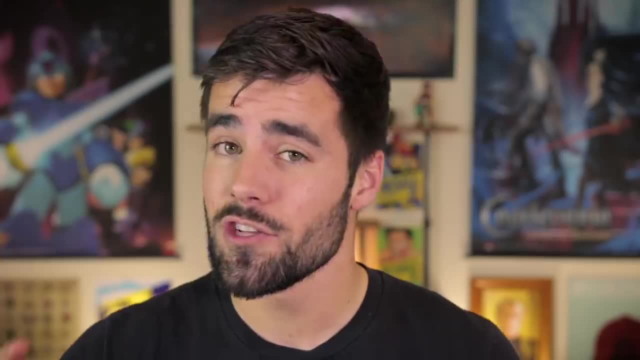 maybe some of you math wizzes out there could do this kind of a problem in your sleep, but it's also possibly the case that you don't have a really good idea of how to solve a really firm grasp on either summation or fractional exponents. So when you're working, 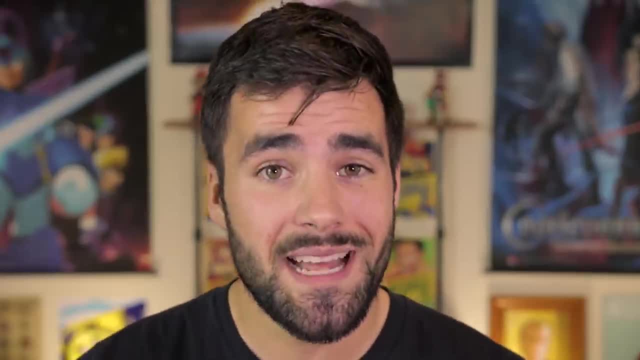 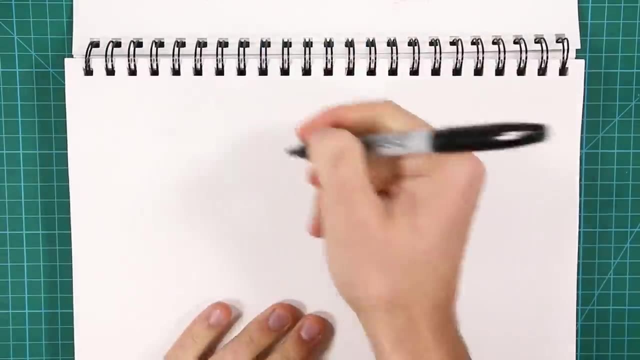 a problem that combines the two of them, you might get stuck. So, assuming that's the case, let's break this problem into two simpler problems that each focus on just one of the underlying concepts. First, let's create a simpler summation problem that just gets rid. 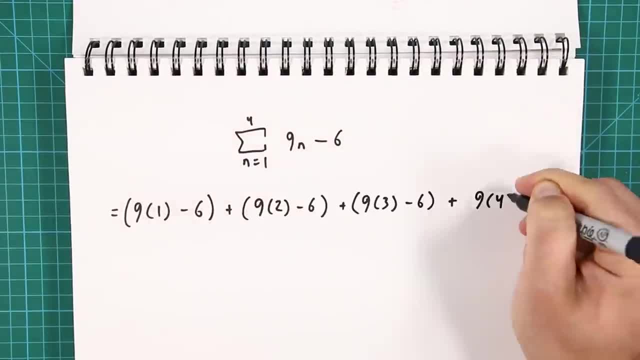 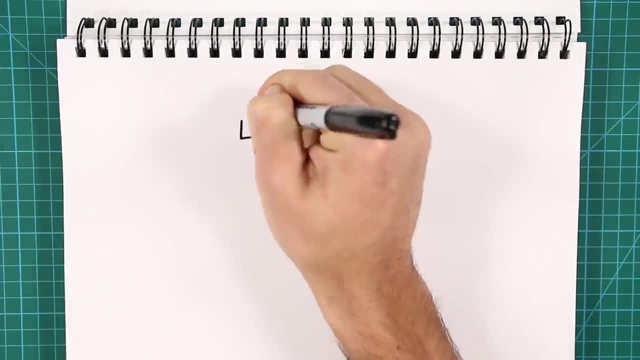 of that fractional exponent altogether. Now all we have to do is evaluate that expression four times and then add up the answers, which gets us to a final answer of 66.. And now let's move on to the fractional exponent. Now I'm going to go pretty quick here, because this: 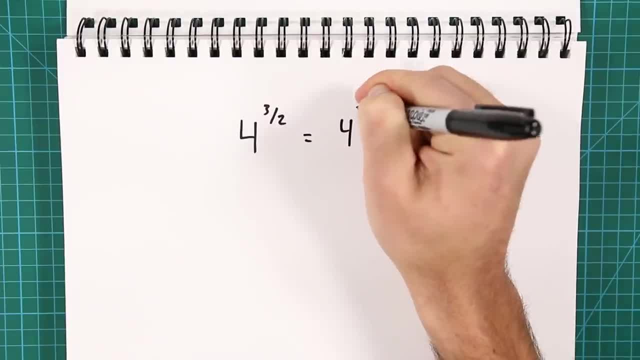 is not a lesson on fractional exponents. I'm going to go pretty quick here, because this is not a lesson on fractional exponents. But essentially you can rewrite this as four to the power of three times the power of one half, And then you can rewrite that again to the square root of four to the power of. 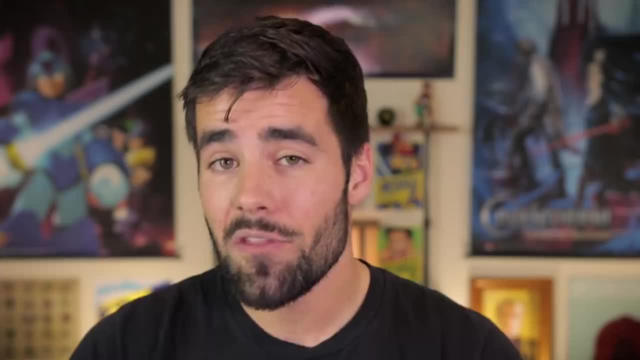 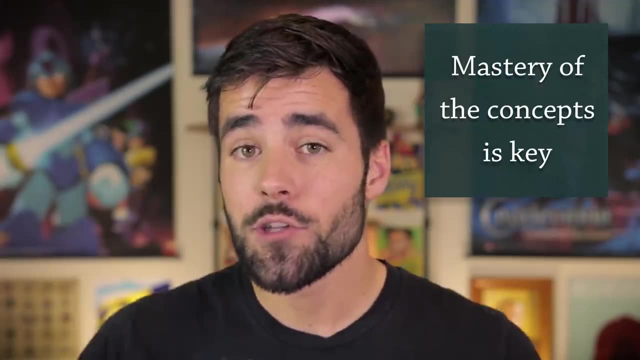 three And once you evaluate that you get an answer of eight. Now the whole point of working these simpler single concept problems is to master the underlying concept or operation that you're working on here. So if you solve a few and you still don't feel really confident, 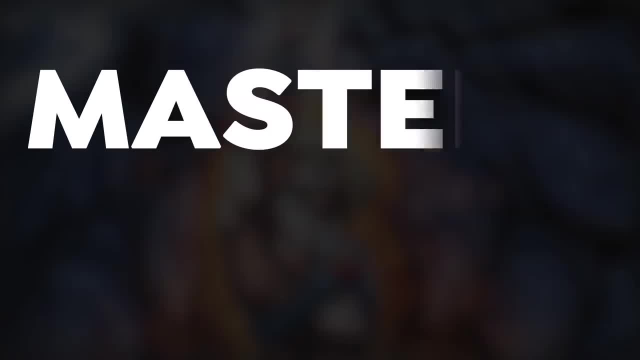 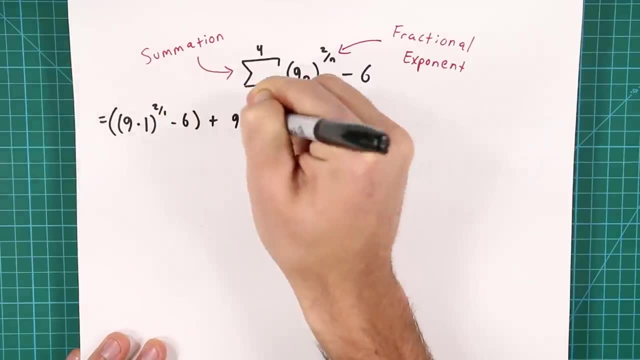 on that concept. keep working it until you do. Remember, mastery means not being able to get it wrong, not just getting it right once. Anyway, once you've mastered those underlying components in an isolated setting, now you can come back to the more complicated. 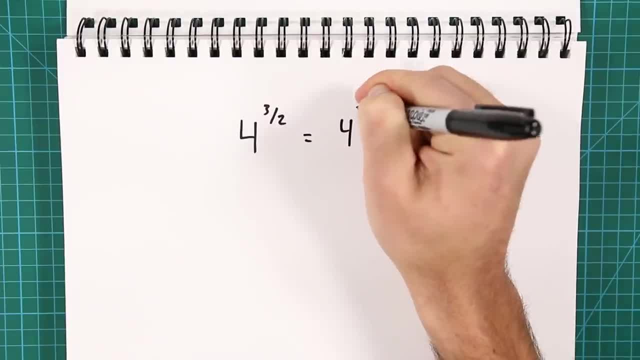 is not a lesson on fractional exponents. I'm going to go pretty quick here, because this is not a lesson on fractional exponents. But essentially you can rewrite this as four to the power of three times the power of one half, And then you can rewrite that again to the square root of four to the power of. 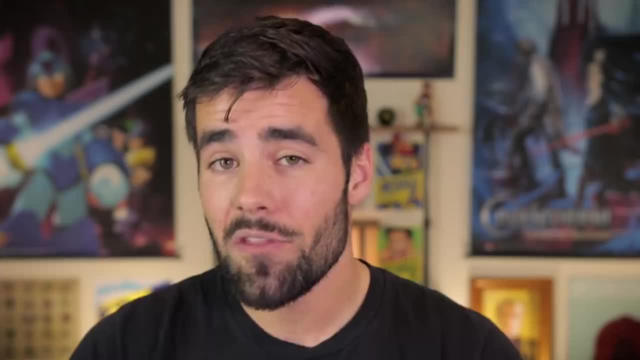 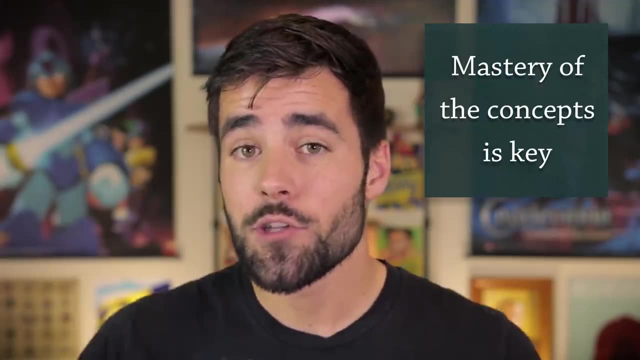 three And once you evaluate that you get an answer of eight. Now the whole point of working these simpler single concept problems is to master the underlying concept or operation that you're working on here. So if you solve a few and you still don't feel really confident, 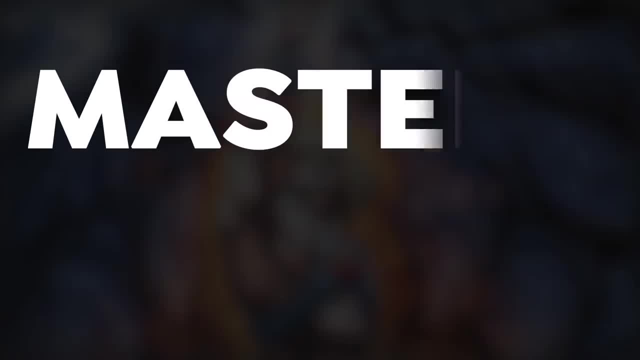 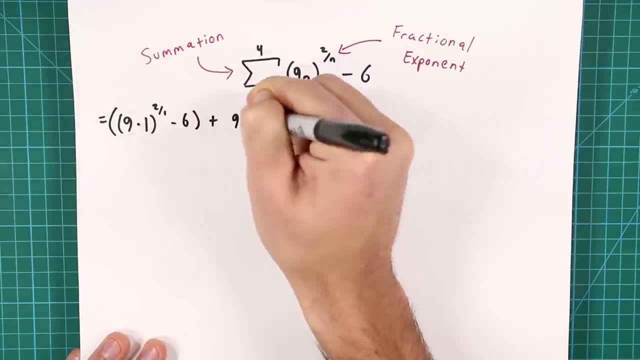 on that concept. keep working it until you do. Remember, mastery means not being able to get it wrong, not just getting it right once. Anyway, once you've mastered those underlying components in an isolated setting, now you can come back to the more complicated. 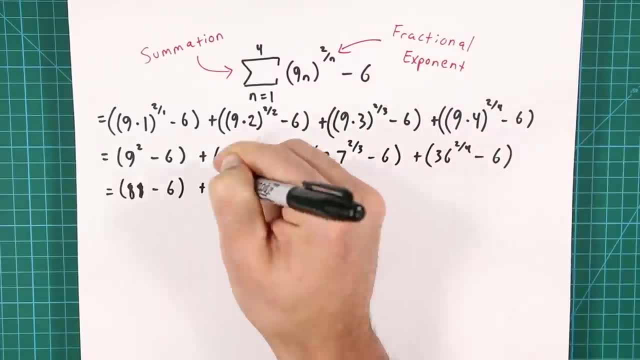 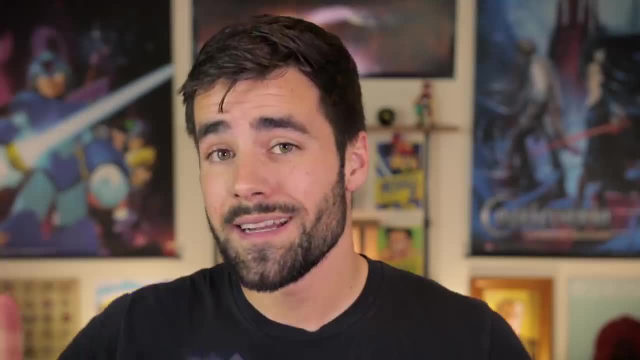 problem that combines them. At this point, you should be able to work those isolated concepts in your sleep, which means that all of your mental processing power can go towards the new and novel problem of how they work in tandem. Now there is one additional way of simplifying tough problems that I want to talk about. 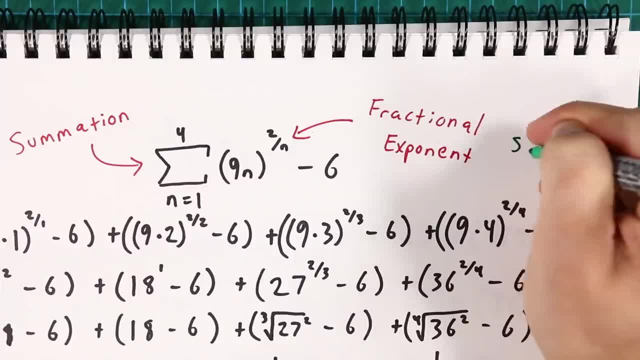 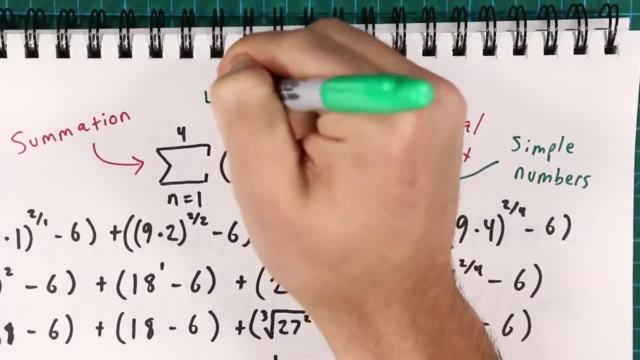 and you might have already guessed it if you paid really close attention to the examples- I didn't use really complex numbers, I didn't use long numbers, I didn't use decimal points, I didn't use big fractions and I stuck to a low limit on my summation problem. Really, 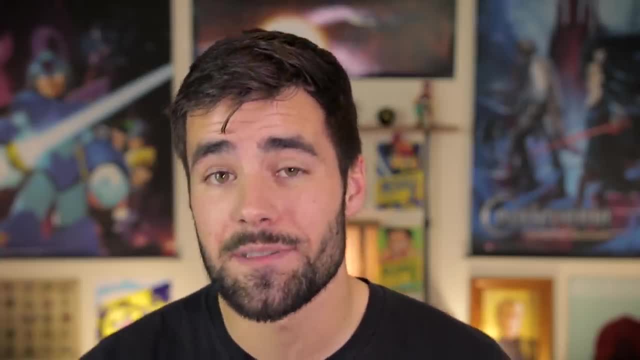 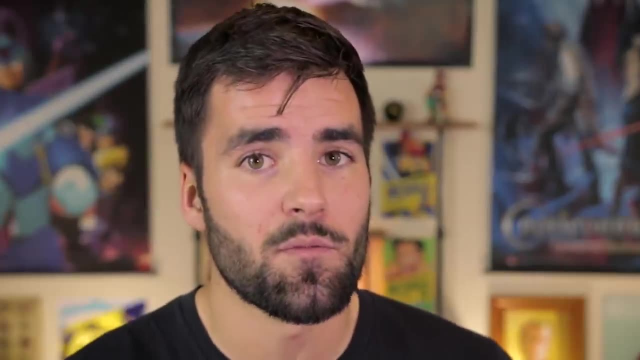 with lots of decimal points can distract your attention away from the concepts and the operations that you're supposed to be practicing. So if you're stuck on a tough problem that has these kinds of numbers go work, a similar problem with really small whole numbers that are easy to add or operate in your head. 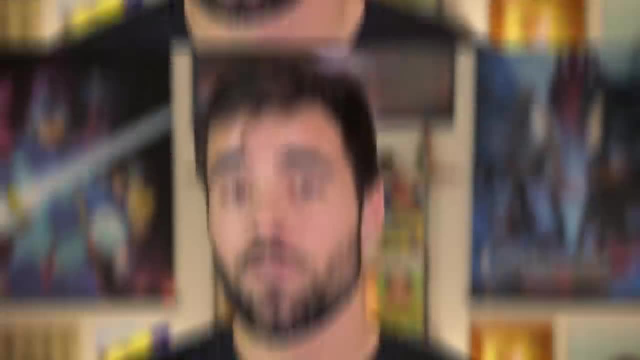 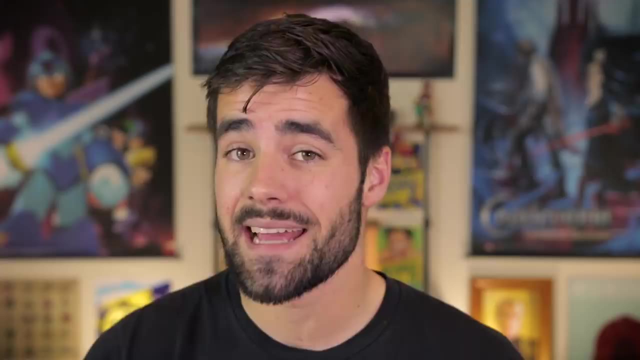 That way you can really zero in on the actual concepts. Of course, sometimes you have too shaky of an understanding of the concepts and operations themselves for you to actually work with them and solve that problem, And in that case it's time to go do some learning. 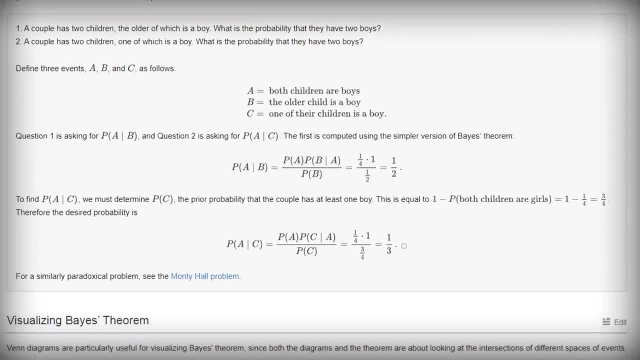 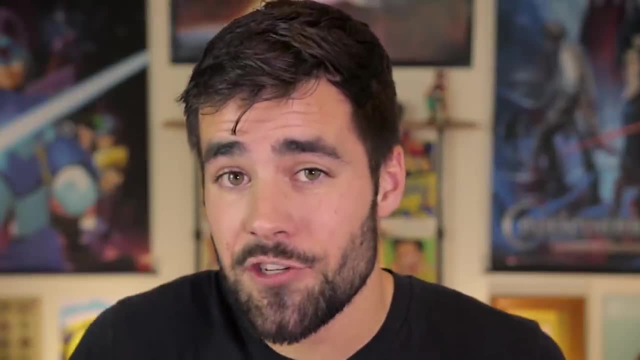 Go, dig into your book, look through your notes or find example problems online that you can follow along with step-by-step, so you can see how people are getting to the solutions using these concepts And, if you need to, you can actually get a step-by-step solution to the exact problem. 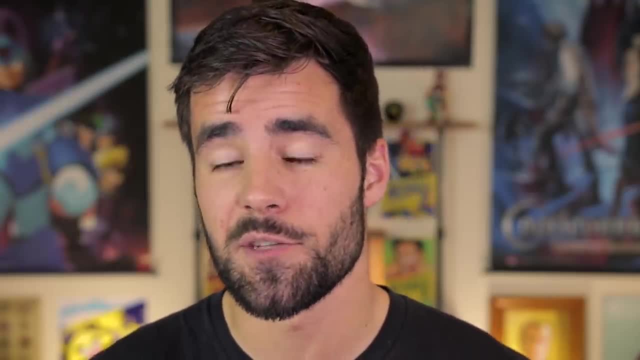 you're working on as well. There are several tools out there that you can use to do this, but the two that I wanna focus on in this video, which are the best ones I've been able to find, are Wolfram, Alpha and Symbolab. 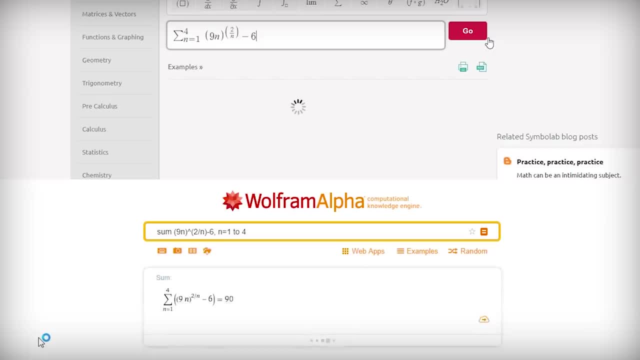 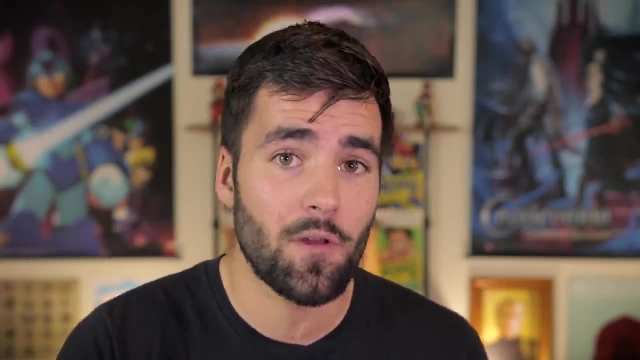 Both of these websites will allow you to type in an equation and get an answer, and also get Alpha and Symbolab that you can follow along with. The difference between the two is that Wolfram Alpha, while being much more powerful and capable, does require you to be part of their paid plan. 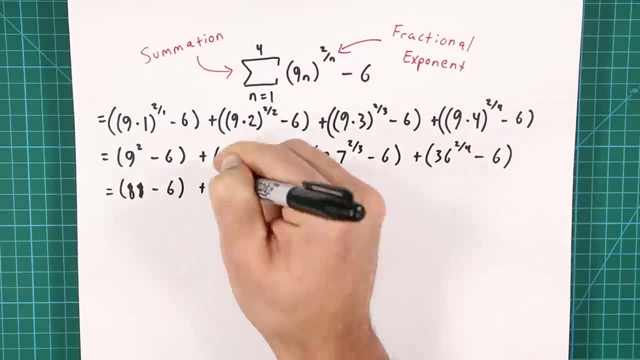 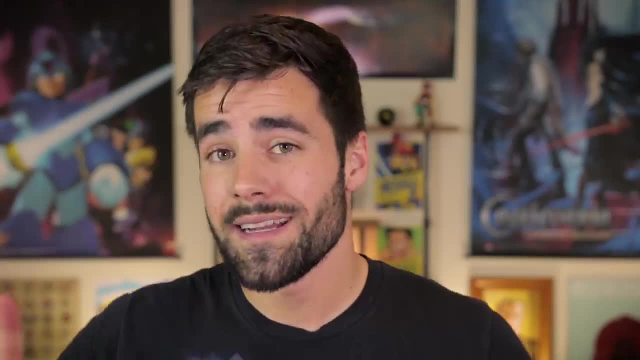 problem that combines them. At this point, you should be able to work those isolated concepts in your sleep, which means that all of your mental processing power can go towards the new and novel problem of how they work in tandem. Now there is one additional way of simplifying tough problems that I want to talk about. 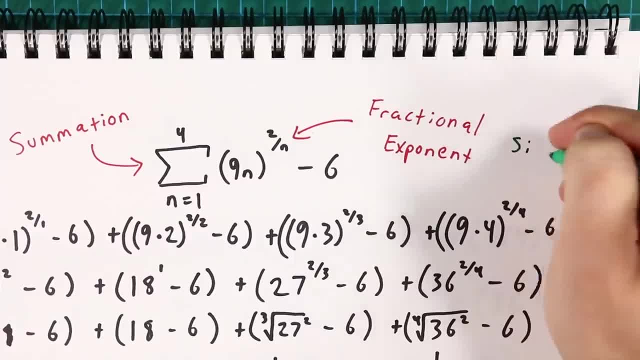 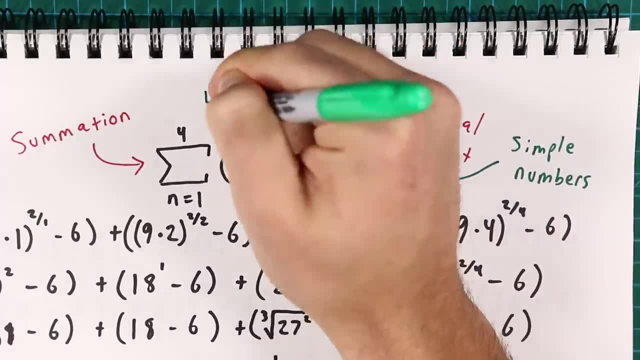 And you might have already guessed it if you paid really close attention to the examples: I didn't use really complex numbers, I didn't use long numbers, I didn't use decimal points, I didn't use big fractions And I stuck to a low limit on my summation problem. Really, 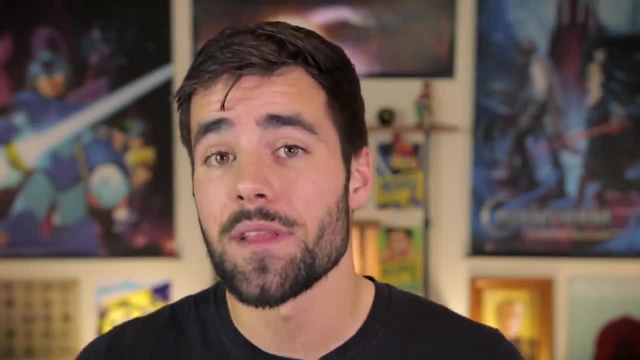 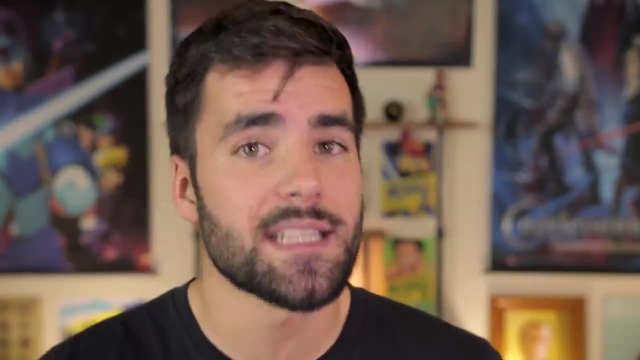 complex big numbers with lots of decimal points can distract your attention away from the concepts and the operations that you're supposed to be practicing. So if you're stuck on a tough problem that has these kinds of numbers go work, a similar problem with really small whole numbers that are easy to add or operate in your head, That way you can really 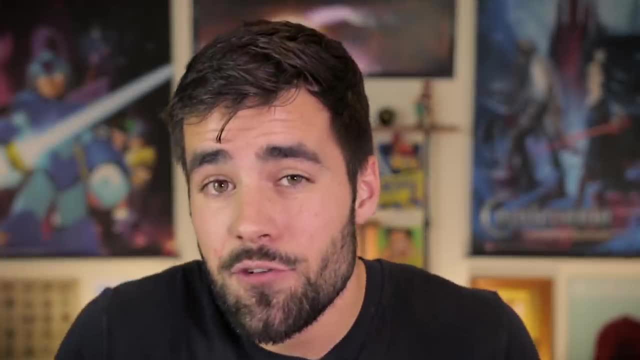 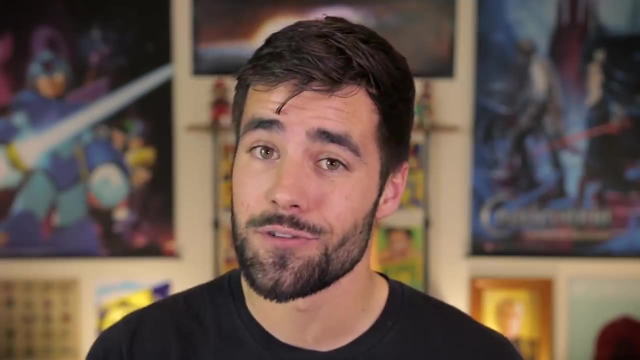 zero in on the actual concepts. Of course, sometimes you have too shaky of an understanding of the concepts and operations themselves for you to actually work with them and solve that problem, And in that case it's time to go do some learning, Go dig into your book. 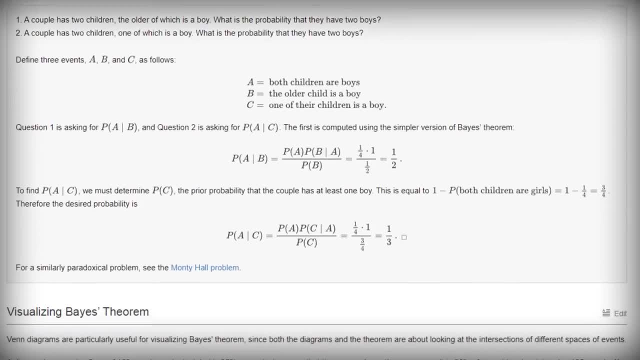 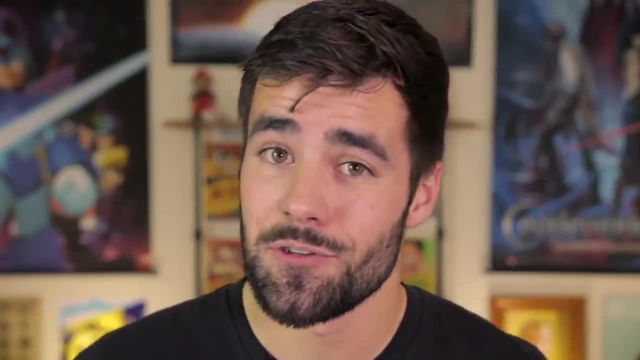 look through your notes. There are some example problems online that you can follow along with step-by-step, so you can see how people are getting to the solutions using these concepts And, if you need to, you can actually get a step-by-step solution to the exact problem you're working. 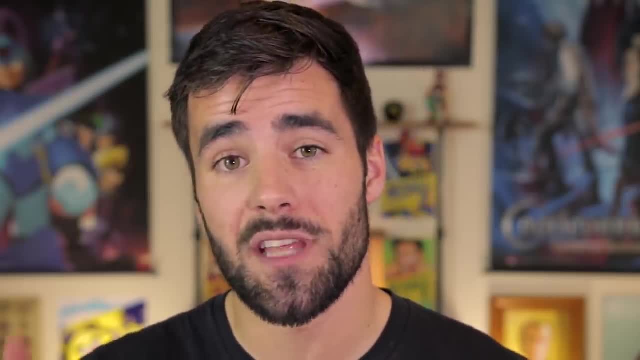 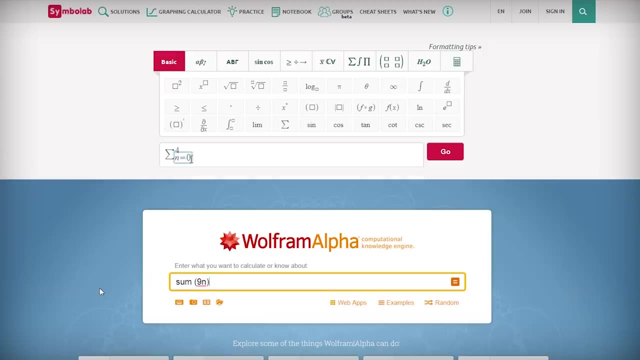 on as well. There are several tools out there that you can use to do this, but the two that I want to focus on in this video, which are the best ones I've been able to find, are Wolfram Alpha and Symbolab. Both of these websites will allow you to type in an equation. 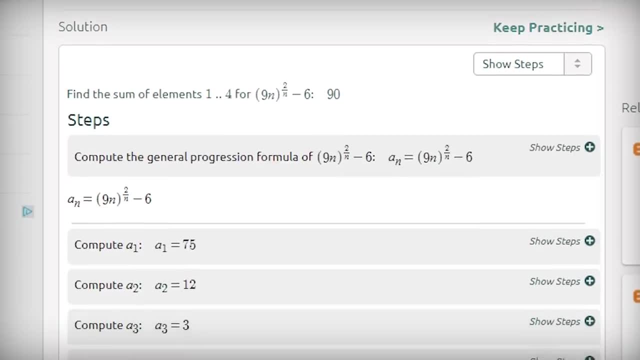 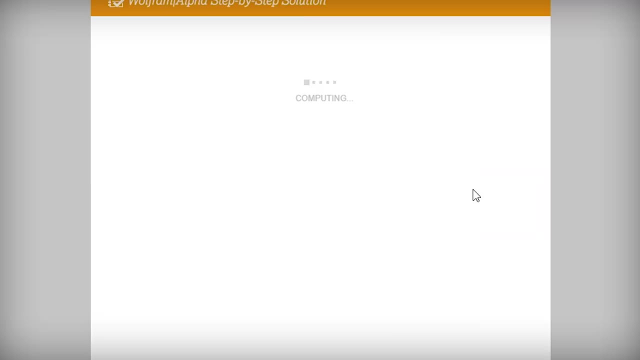 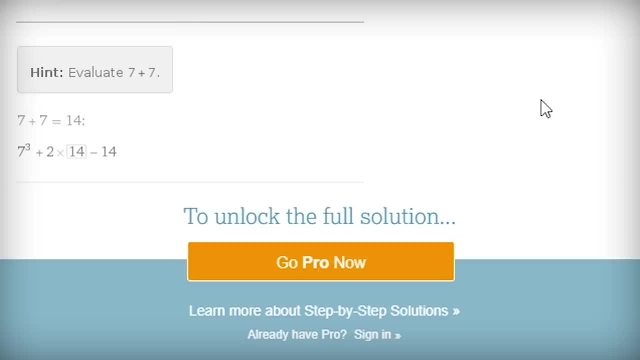 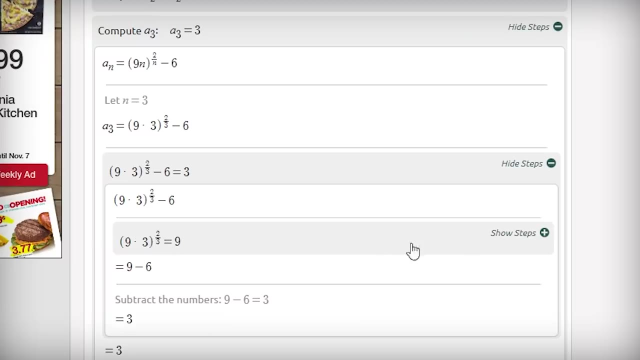 be part of their paid plan if you want to get those step-by-step solutions. By contrast, while I found that typing in equations into Symbolab was a little bit slower and less intuitive than it is with Wolfram Alpha, their step-by-step solutions are free, Regardless. 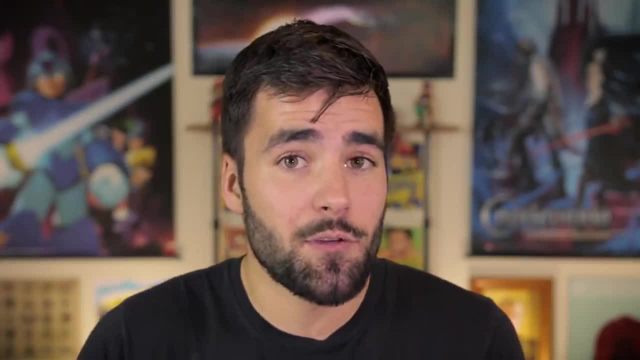 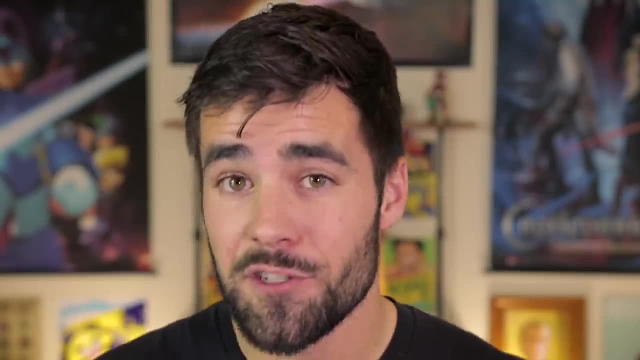 of the tool that you choose to use here. the underlying point is that sometimes it can be useful to see a step-by-step solution for a problem you're stuck on. But there are two very important caveats here. First and foremost, before you go running off to find a solution, 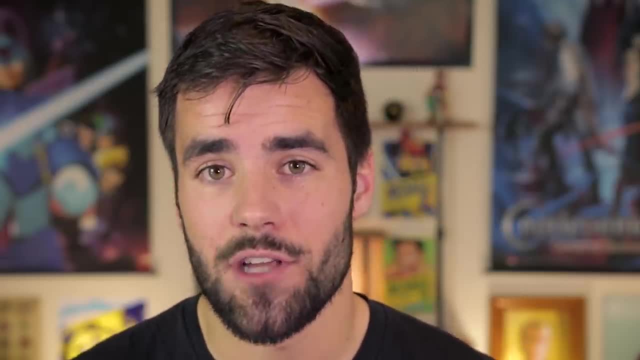 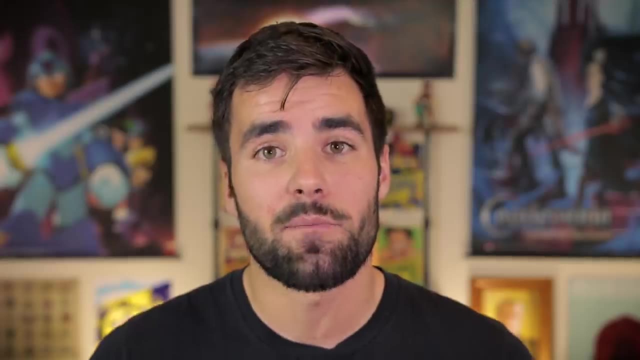 ask yourself Honestly: have I pushed my brain to the limit trying to solve this problem first? Expending the mental effort required to solve the problem yourself is going to stretch your capabilities. It's gonna make you a better mathematician in a way that just looking through solutions won't. 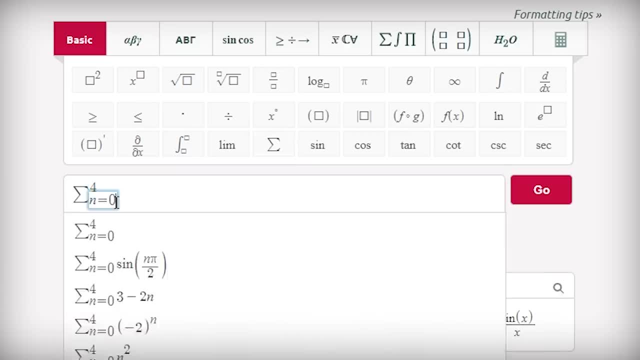 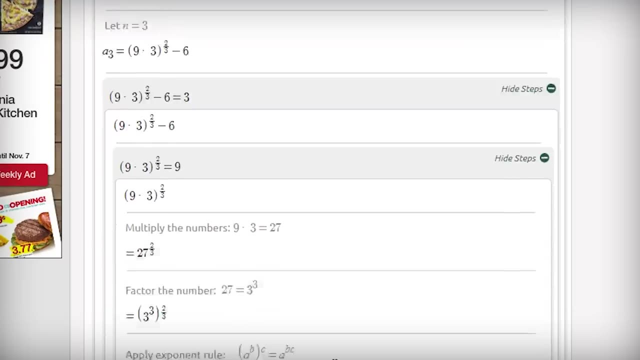 if you wanna get those step-by-step solutions. By contrast, while I found that typing in equations into Symbolab was a little bit slower and less intuitive than it is with Wolfram Alpha, their step-by-step solutions are free, Regardless of the tool that you choose to use here. 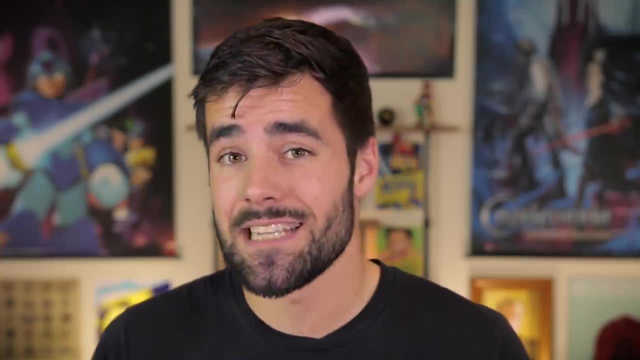 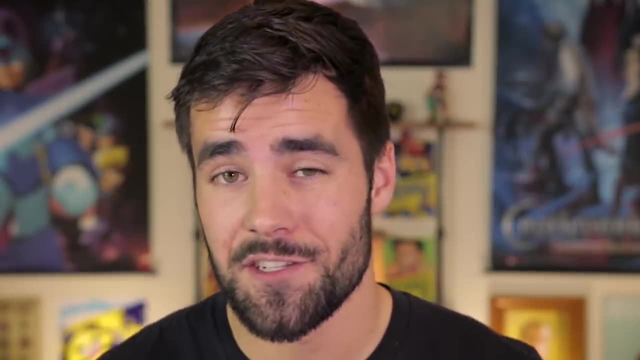 the underlying point is that sometimes it can be useful to see a step-by-step solution for a problem you're stuck on, But there are two very important caveats here. First and foremost, before you go running off to find a solution, ask yourself honestly, have I pushed my brain? 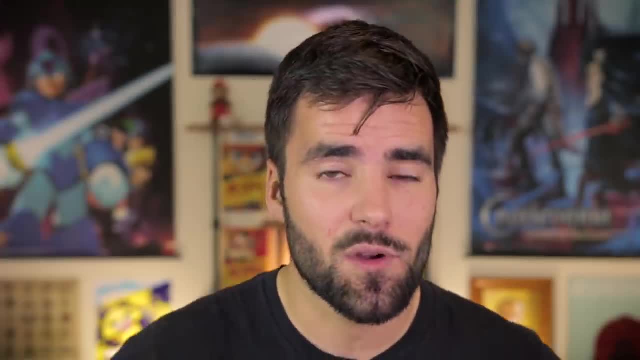 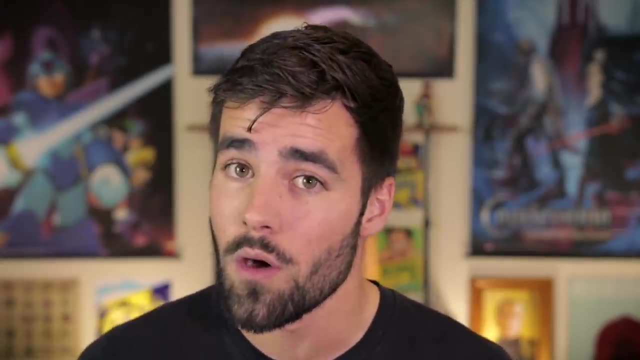 to the limit trying to solve this problem first. Expending the mental effort required to solve the problem yourself is going to stretch your capabilities. It's gonna make you a better mathematician in a way that just looking through solutions won't. Now, if you do need to look up a solution, that's fine. 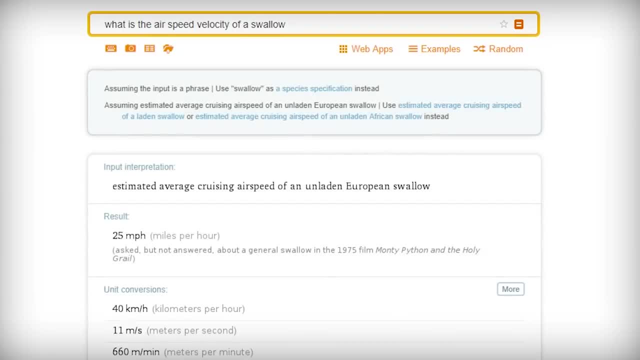 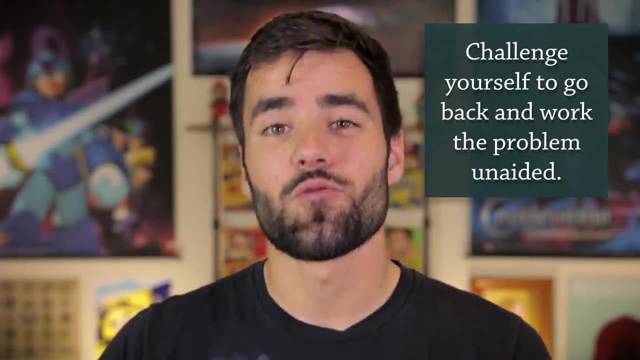 Look it up, follow the steps and make sure you understand how the answer was arrived at. But once you've done that, challenge yourself to go back and rework the problem without looking at that reference. It is really important to stay vigilant about this. 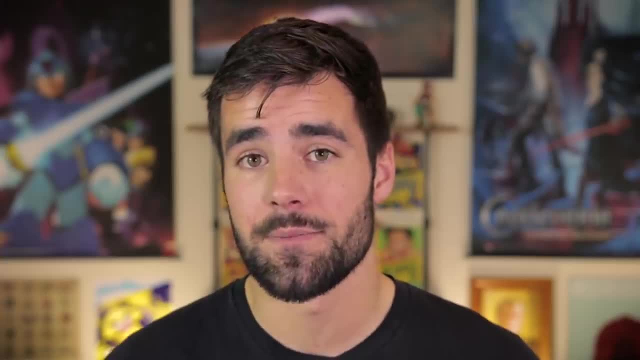 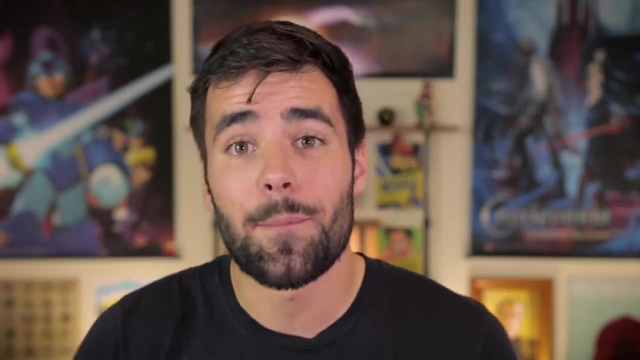 because if you wanna get better at it and better at math, the whole point is to master the concepts that you're working with. The danger that comes with looking up solutions is that with math it's really easy to follow along with a step-by-step solution and comprehend what's going on. 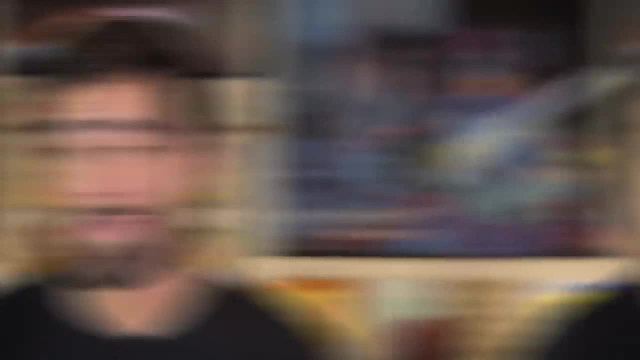 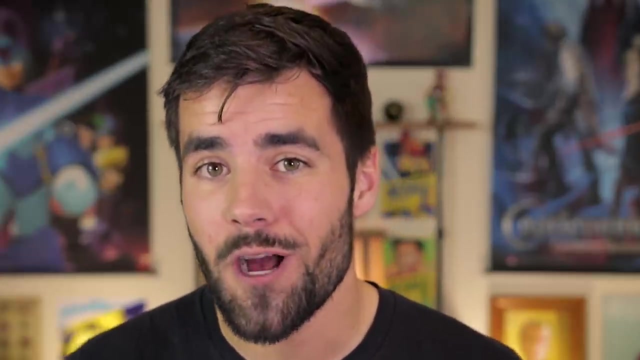 But that is very different than being able to do it on your own. And that brings me to my final tip for you, and this is especially important for anybody in a math class working through assigned homework: Don't rush when you work through math problems. 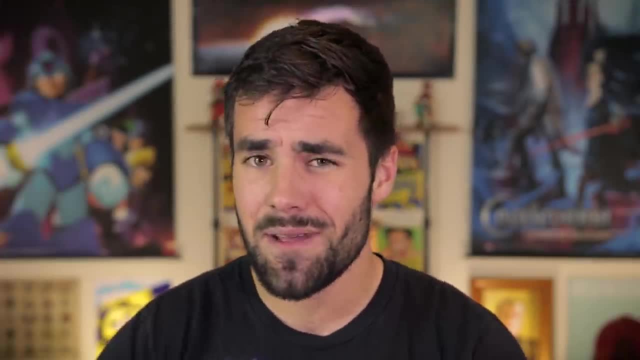 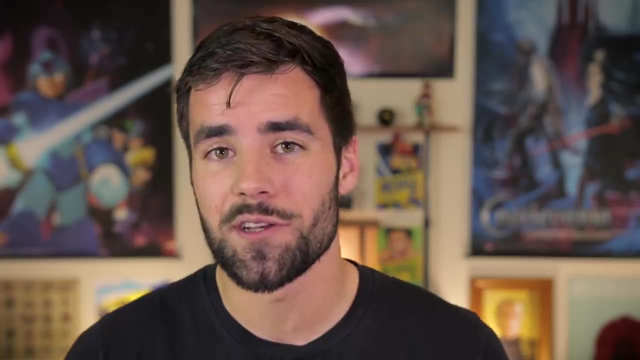 I know it's really tempting to try to work through homework as fast as you can and heck, I even made a video about it pretty recently. But with math and science and any sort of really complex subject, especially rushing is only going to hurt you down the road. 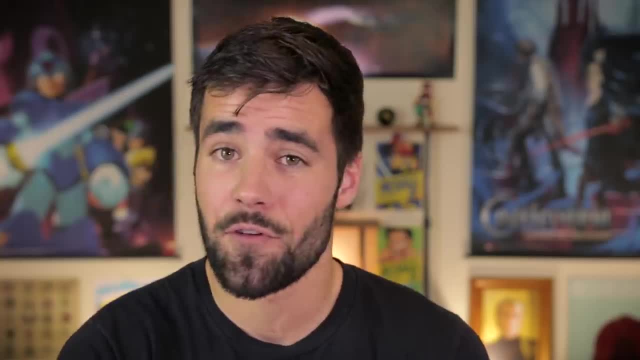 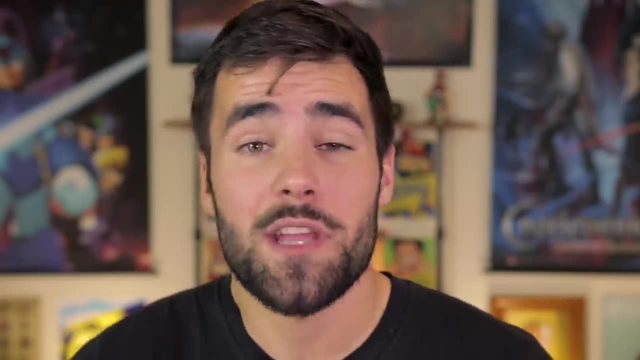 Because when you rush, you don't master the concepts. You just brute force your way to answers, or you look things up, or you otherwise kinda cheaty face your way to a completed homework assignment And later on, when you're sitting in a testing room, 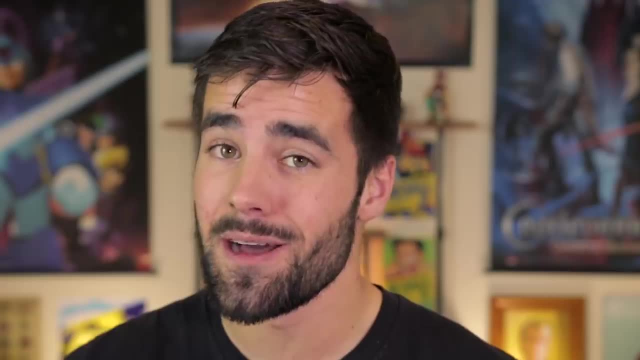 or you have to apply what you've learned in the real world. you are gonna get a harsh lesson about exactly what it is you don't know. So let's recap here. If you wanna get better at math and you wanna improve your ability, 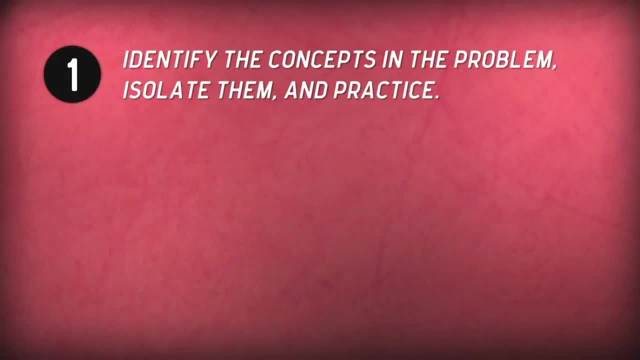 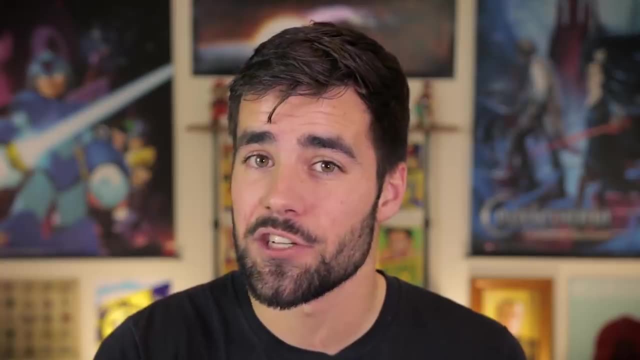 to solve those really tough problems. first identify the combination of concepts or operations being used in a problem and then isolate them. Work simpler problems that use just one and then master each concept. You can also simplify the problem by leaving the combination of concepts intact. 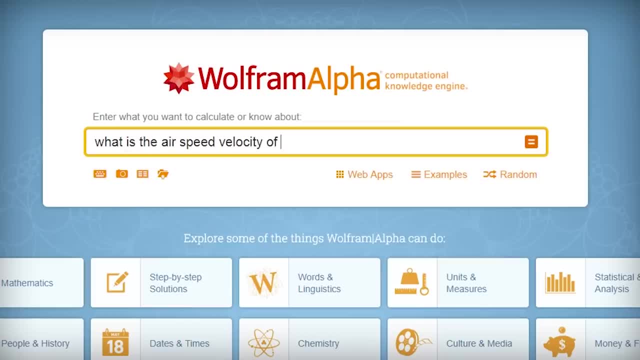 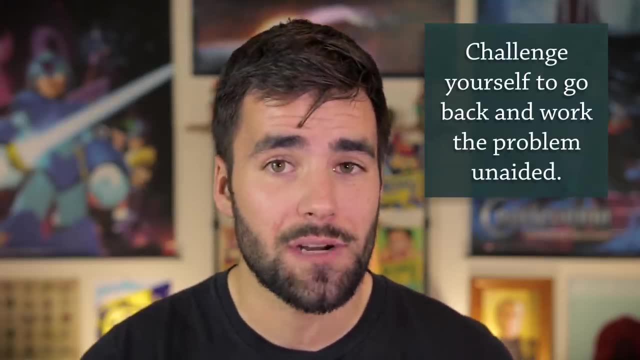 Now, if you do need to look up a solution, that's fine. Look it up, follow the steps and make sure you understand how the answer was arrived at. But once you've done that, challenge yourself to go back and rework the problem. 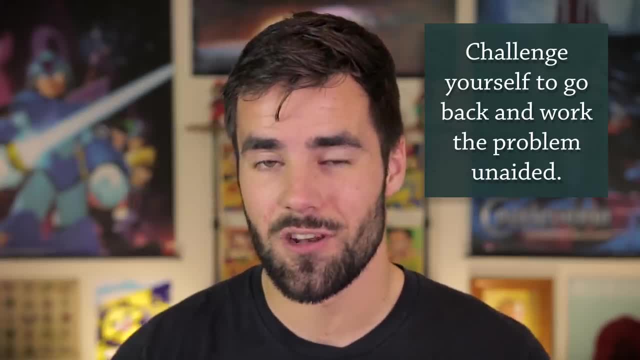 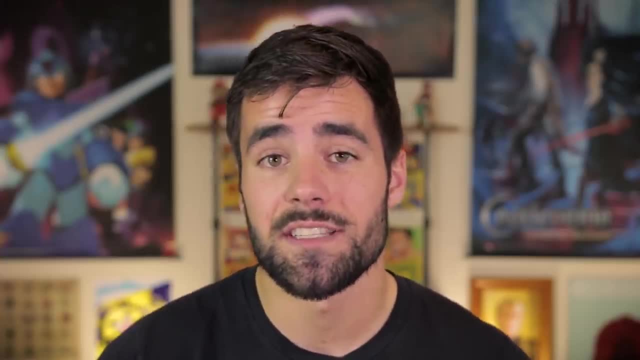 without looking at that reference. It is really important to stay vigilant about this, because if you wanna get better at math, the whole point is to master the concepts that you're working with. The danger that comes with looking up solutions is that with math, it's really easy to follow along. 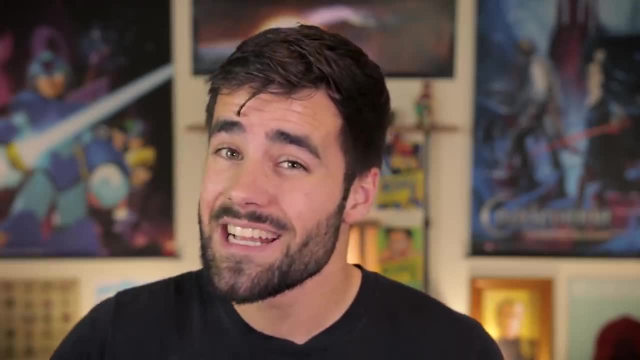 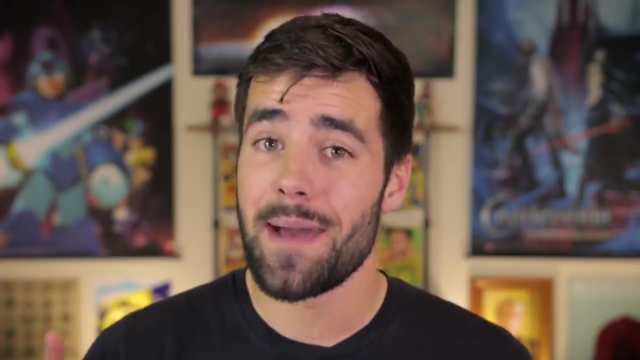 with a step-by-step solution and comprehend what's going on, But that is very different than being able to do it on your own. And that brings me to my final tip for you, and this is especially important for anybody in a math class working through assigned homework. 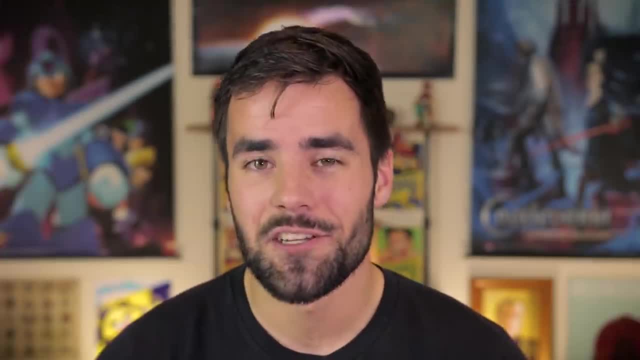 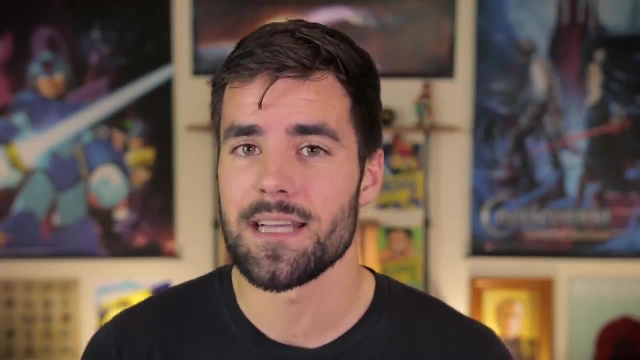 Don't rush when you work through math problems. I know it's really tempting to try to work through homework as fast as you can and heck, I even made a video about it pretty recently- But with math and science and any sort of really complex subject especially, 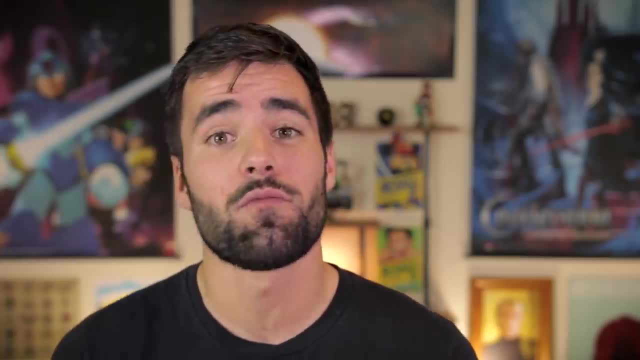 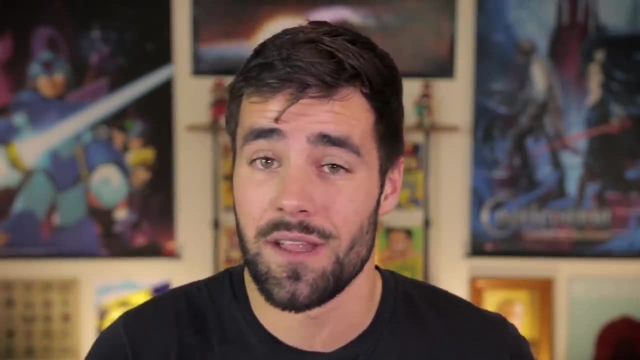 rushing is only going to hurt you down the road, because when you rush you don't master the concepts. You just brute force your way to answers, or you look things up, or you otherwise kinda cheaty face your way to a completed homework assignment And later on when you're sitting in a testing room, 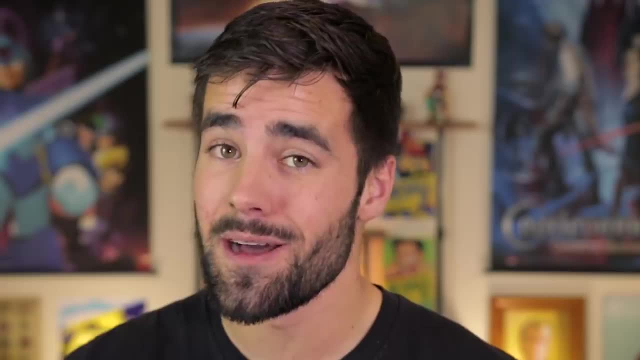 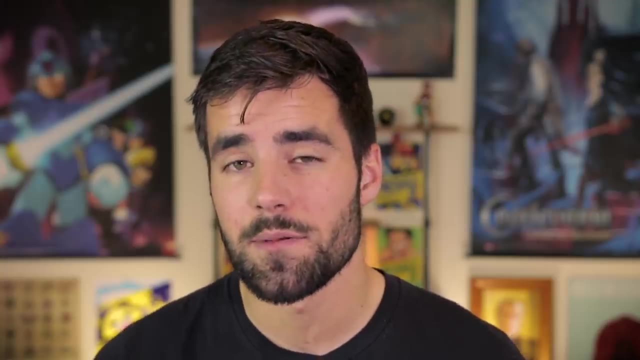 or you have to apply what you've learned in the real world. you are gonna get a harsh lesson about exactly what it is you don't know. So let's recap here: If you wanna get better at math and you wanna improve your ability to solve those really tough problems, 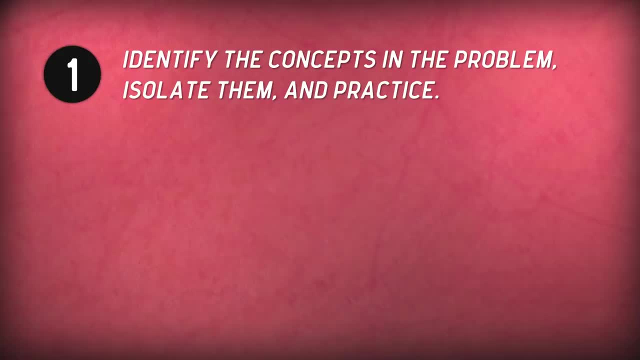 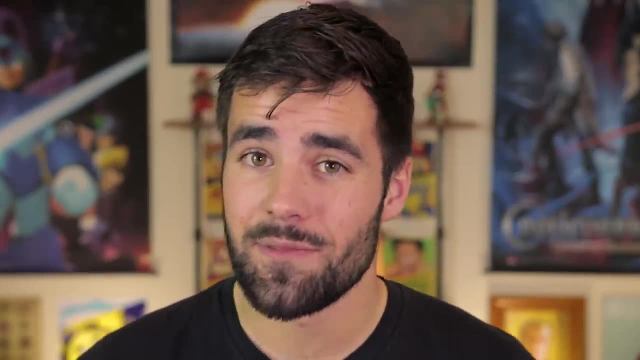 first identify the combination of concepts or operations being used in a problem and then isolate them. Work simpler problems that use just one and then master each concept. You can also simplify the problem by leaving the combination of concepts intact, but swapping in smaller, easier-to-handle numbers. 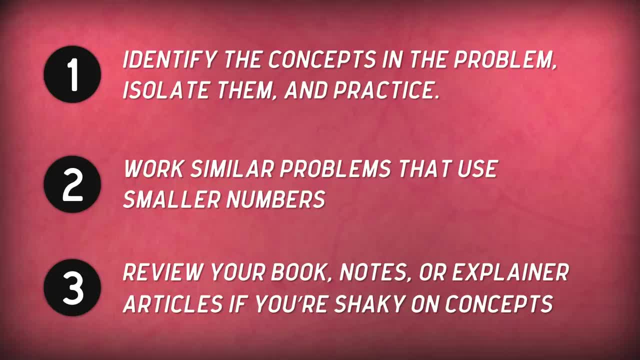 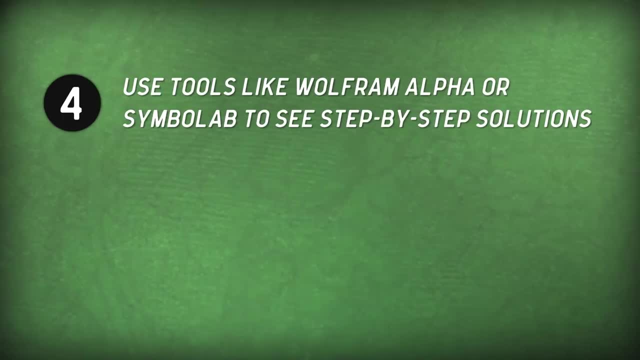 If you need help with the concepts themselves, go to your book or an explainer article online, look up sample problems or use a tool like Wolfram, Alpha or Symbolab to get step-by-step solutions to the problem you're working on. And finally, don't rush through your homework assignments. 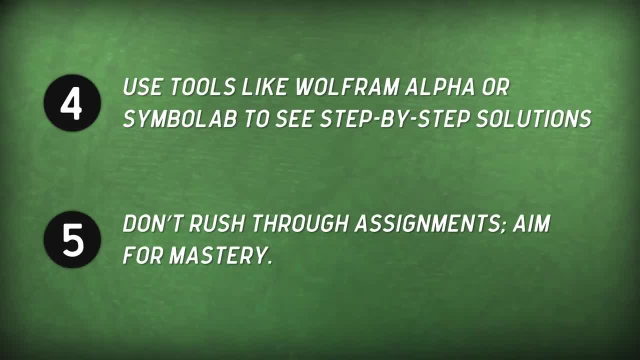 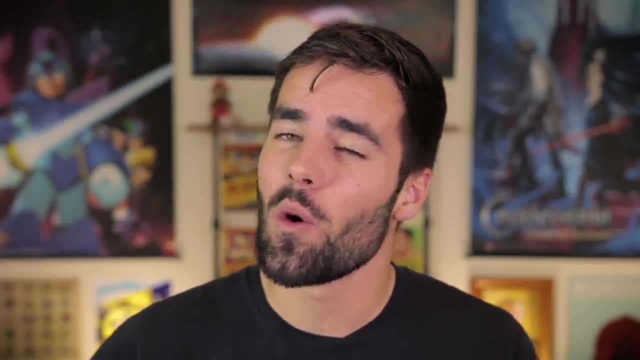 Make sure that you're focusing intently on mastering the concepts, not just finishing. Hopefully, these tips will give you the confidence to tackle some really tough math problems and to expand your math skillset. And on that note, I wanna leave you with a quote. 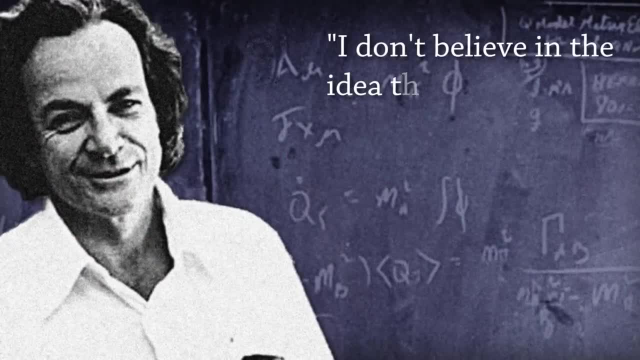 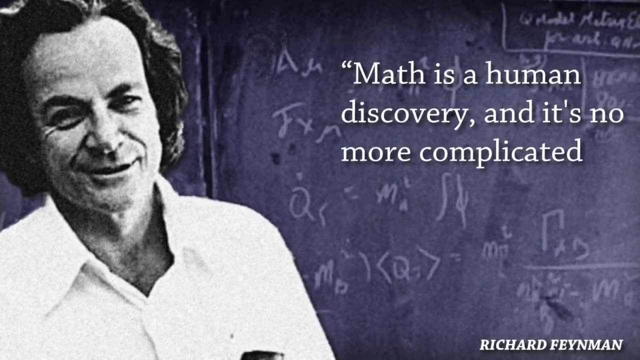 from the great physicist Richard Feynman, who said: "'I don't believe in the idea "'that there are few peculiar people "'capable of understanding math "'and the rest of the world is normal. "'Math is a human discovery, "'and it's no more complicated than humans can understand'". 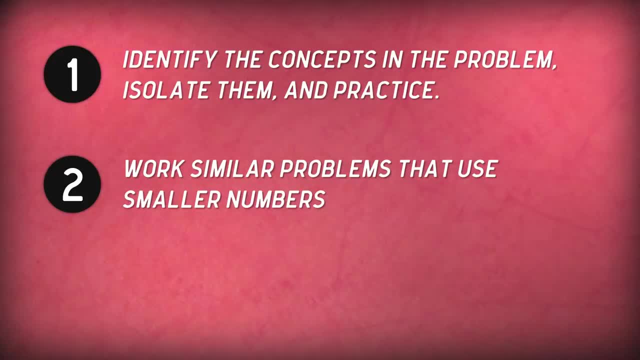 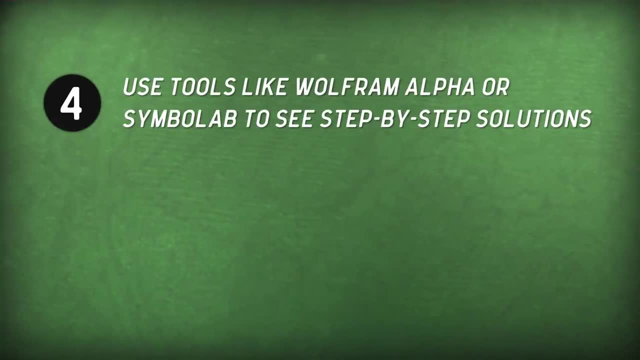 but swapping in smaller easier to handle numbers. If you need help with the concepts themselves, go to your book or an explainer article online, look up sample problems or use a tool like Wolfram, Alpha or Symbolab to get step-by-step solutions. 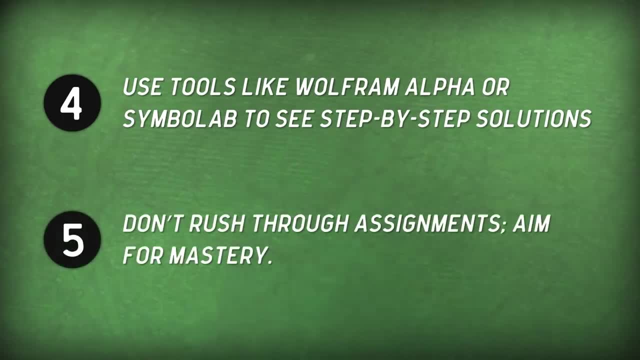 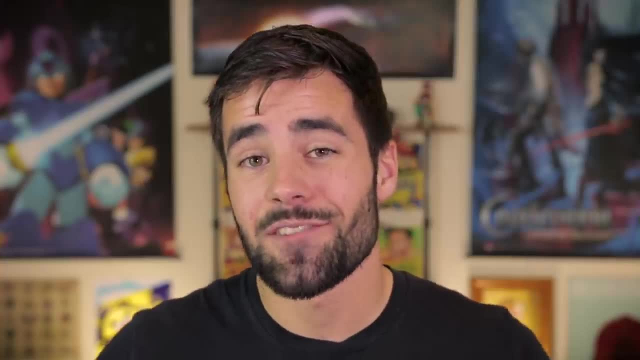 to the problem you're working on. And finally, don't rush through your homework assignments. Make sure that you're focusing intently on mastering the concepts just finishing. Hopefully, these tips will give you the confidence to tackle some really tough math problems. 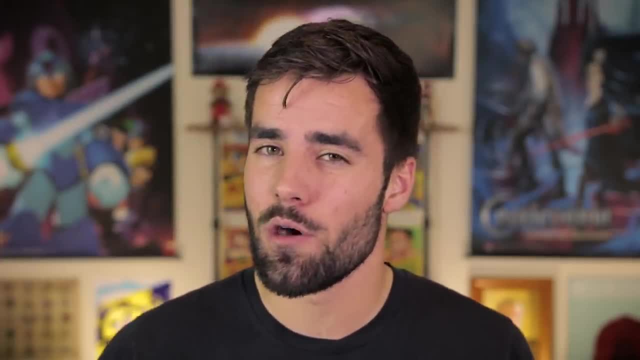 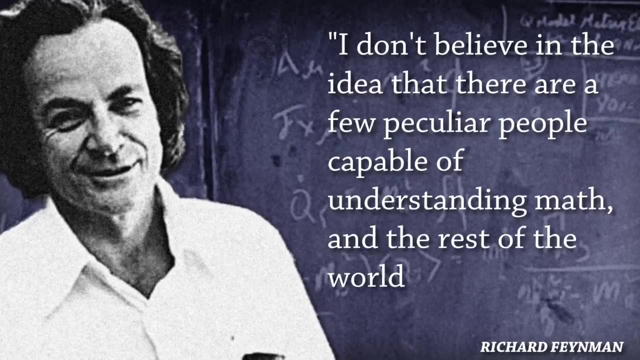 and to expand your math skillset. And on that note, I wanna leave you with a quote from the great physicist Richard Feynman, who said: I don't believe in the idea that there are few peculiar people capable of understanding math and the rest of the world is normal. 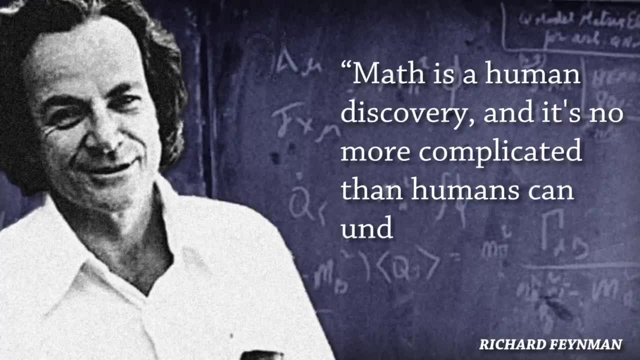 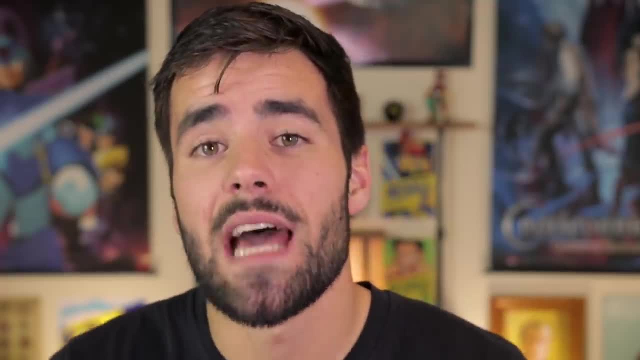 Math is a human discovery and it's no more complicated than humans can understand. The bottom line is this: Ultimately, your ability to get good at math- and anything else for that matter- starts with having the confidence to approach it And as you solve problems. 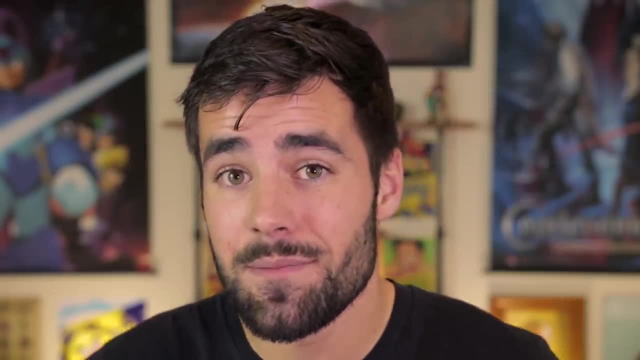 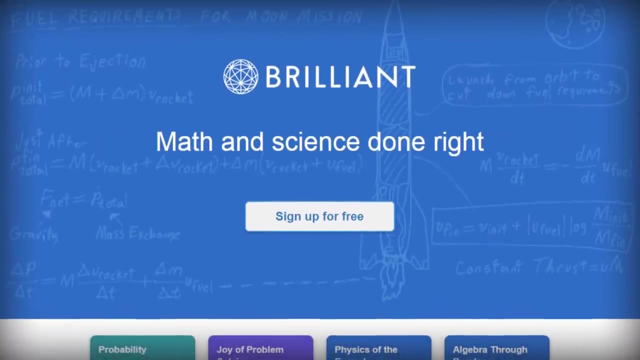 and make mental breakthroughs, your confidence is going to naturally increase. It becomes a self-sustaining cycle. If you're interested in starting the cycle of learning now, a great place to begin your journey is at Brilliant, a learning platform that uses hands-on problem solving. 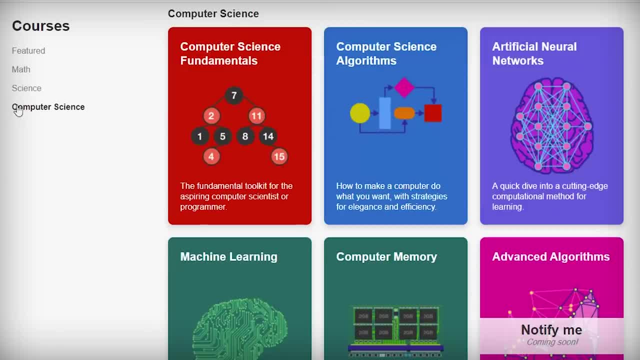 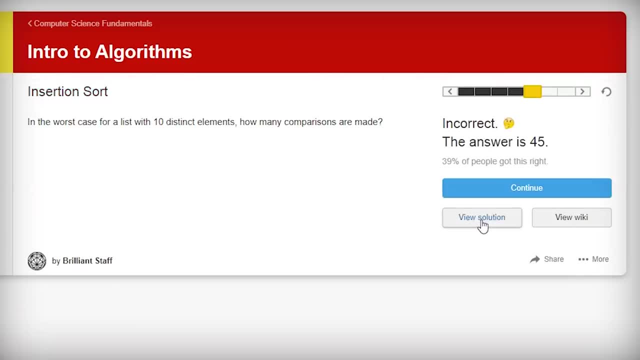 as a basis to help you learn math science and computer science really effectively. I'm actually taking their Computer Science Fundamentals course right now and as I was going through the first section on algorithms, the quiz questions they gave me forced me to learn new math I had never learned before. 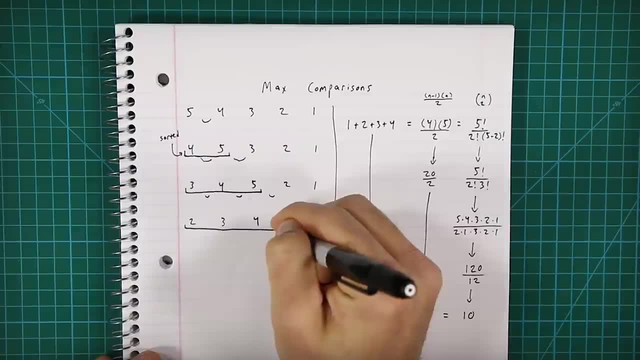 I had to dig into wikis and example problems and eventually I had to get out a sheet of notebook paper and literally draw out algorithms step-by-step so I could understand what was going on. This process provided me with a much more intense 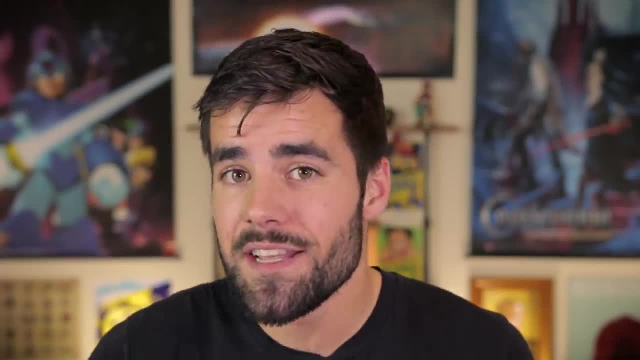 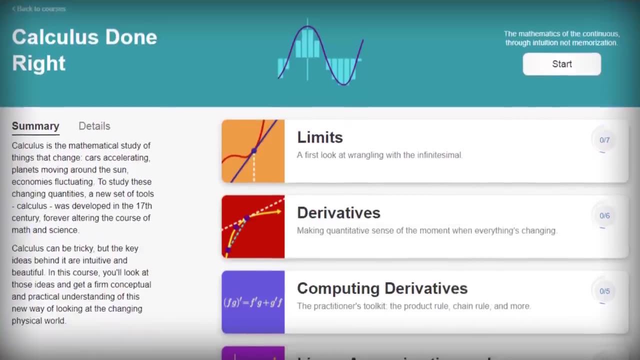 and effective learning experience than I got sitting through most of my college lectures And these types of challenges that really force you to dig in form the foundation for all of their courses, which include probability, logic, calculus, astronomy, computer memory and more. 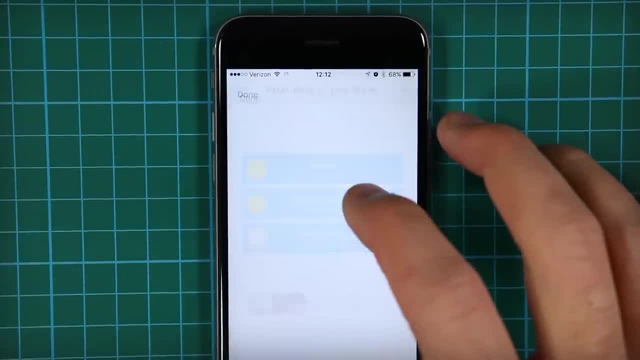 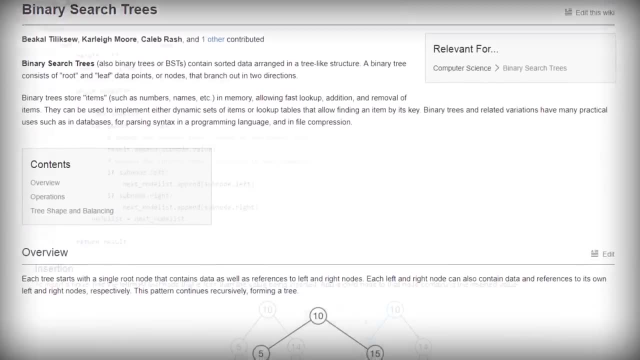 In addition to those structured courses, Brilliant also has weekly challenges that you can use to improve your skills. it has a community where you can talk with other learners, and it has a fantastically detailed and helpful wiki with lots of explanations and examples. 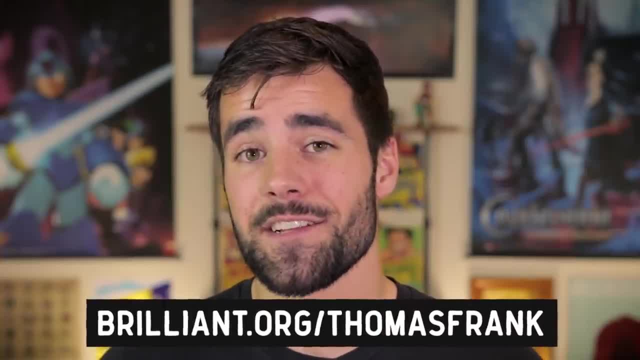 So if you wanna give Brilliant a try, click the link in the description down below and sign up for free to start learning And as a bonus, if you're among the first 200 people to sign up, you'll also get 20% off.